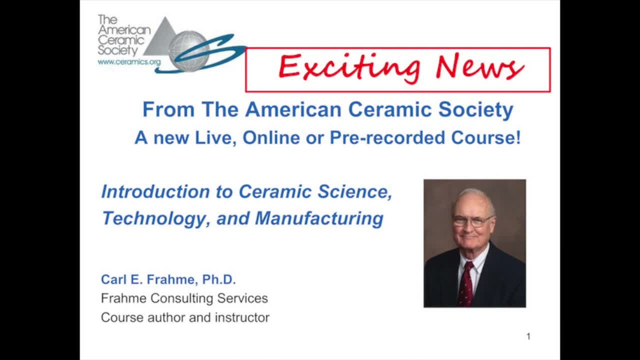 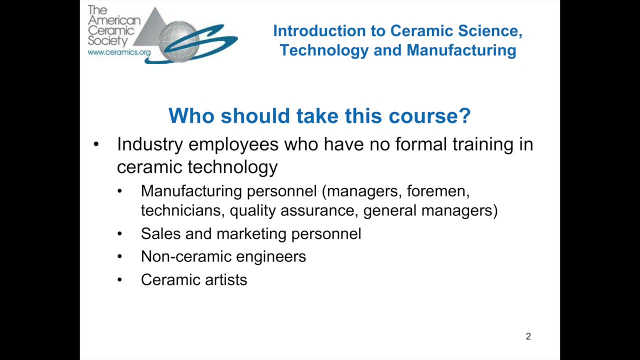 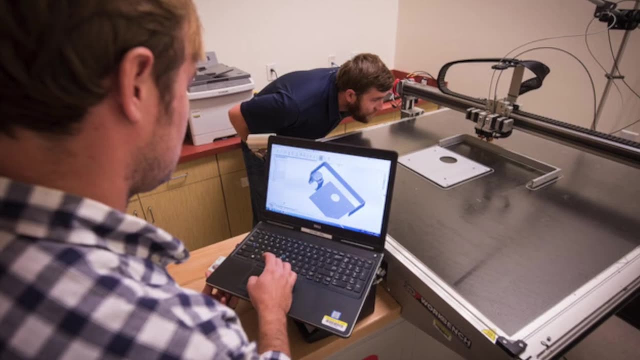 title and the course lives up to that breadth. Are you a candidate for taking this course? Well, if you are in the ceramic industry and have had no formal training in ceramic technology, you could be a candidate, And that includes manufacturing personnel managers. 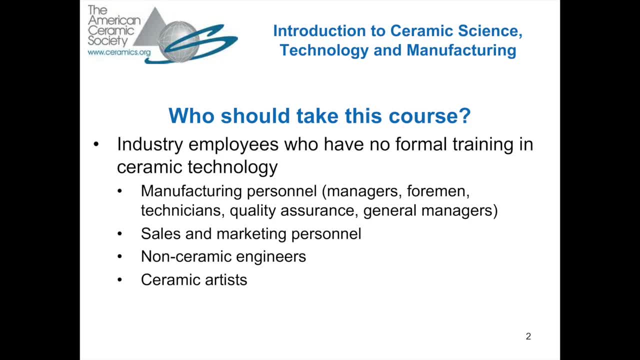 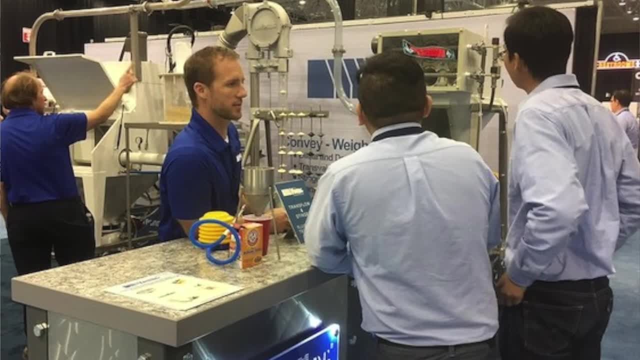 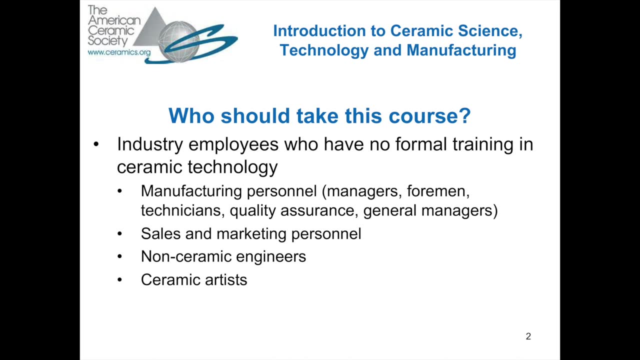 foremen technicians, quality assurance personnel, general managers. It includes sales and marketing personnel who have to speak intelligently to their customers. It includes non-ceramic engineers: mechanical engineers, chemical engineers, civil engineers who have had no formal training per se in ceramic technology. 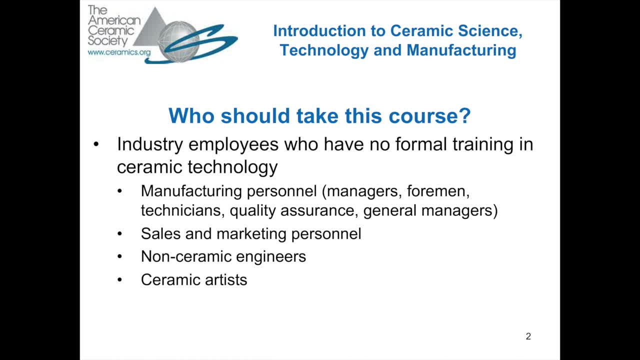 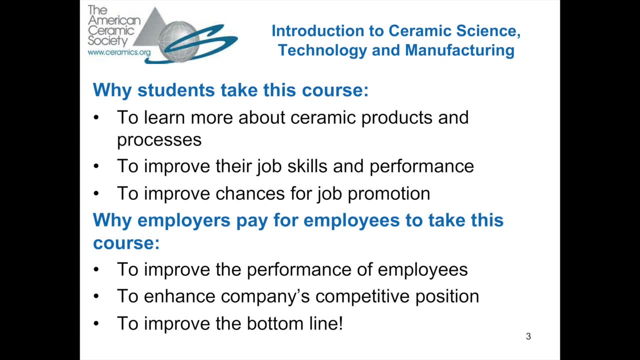 It also includes serious ceramic artists. Why do students sign up for this course? First of all, they want to learn more about ceramic products and processes, which they will do. They want to improve their job skills and performance. That's one of the primary reasons. 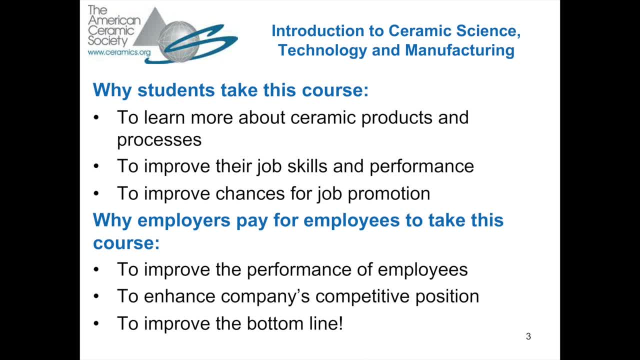 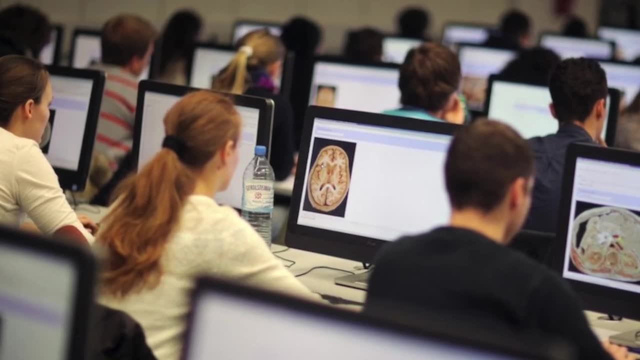 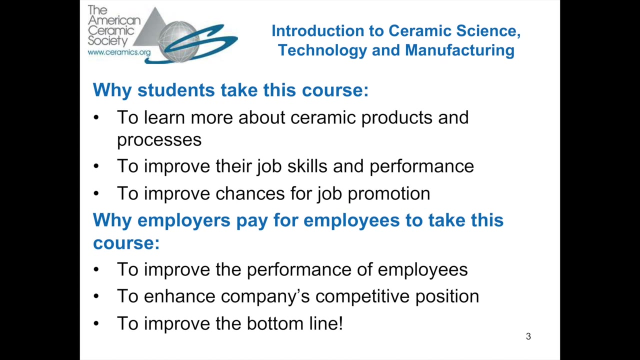 that they sign up, And they also want to improve their chances for promotion. Why do employers pay money for their employees to take this course? They want to improve the performance of their employees. They realize that untrained employees are not as productive. They also want to enhance the company's competitive position in the 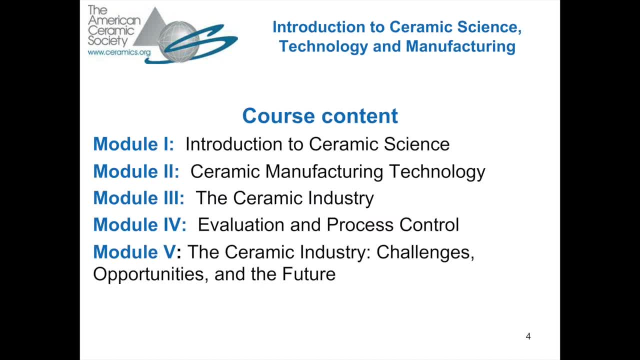 industry and they want to improve the bottom line. The course content is quite extensive. There are five modules. The first module is Introduction to Ceramic Science. You really cannot understand ceramics and their properties and their applications unless you understand the depth of the technology You're going to have a lot of experience with. 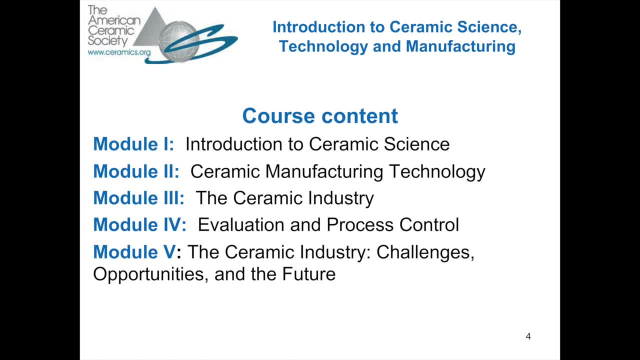 the basics of Ceramic Science. You don't have to have any training in Ceramic Science to take this course. Everything you need is presented in the course. Module 2 is Ceramic Manufacturing Technology: a very extensive look at all the steps used to manufacture ceramics, including glass products. Module 3 is a 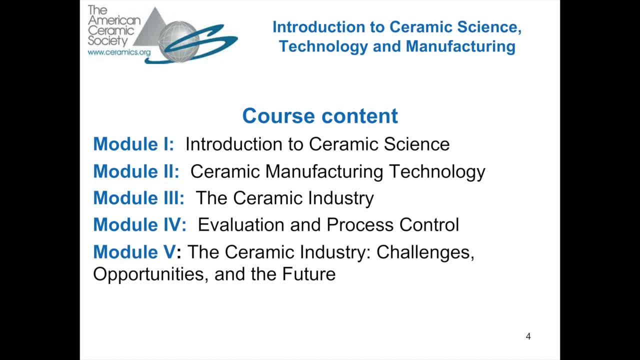 look at five major segments of the ceramic industry. Module 4 is on evaluation and process control: a lesson on measurement of properties of ceramic materials and a very important lesson on statistical process control. The last module looks at challenges and opportunities and the future of this.